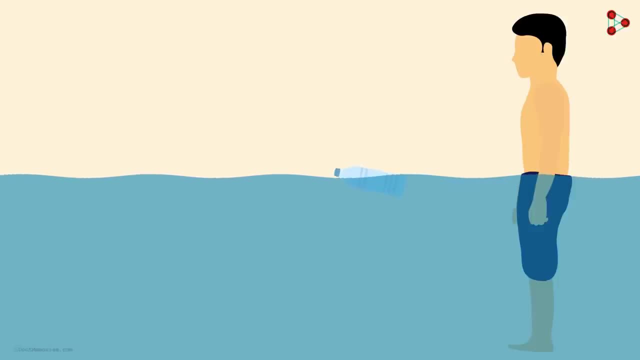 own. I think you can guess why. Now push the bottle deeper inside the fluid. You will feel more force against your hand And when you release the bottle it'll rush back to the surface. It'll come up faster than it came up in the previous case. 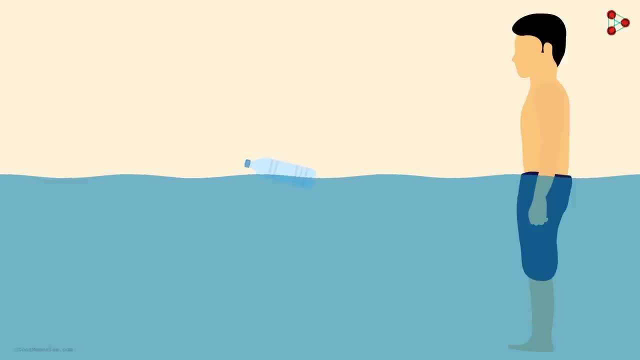 The upward force increases as it's pushed deeper into the fluid, And that's because the pressure also increases as we go deeper into the fluid. This upward force exerted by the water on the bottle is known as upthrust or the buoyant force. 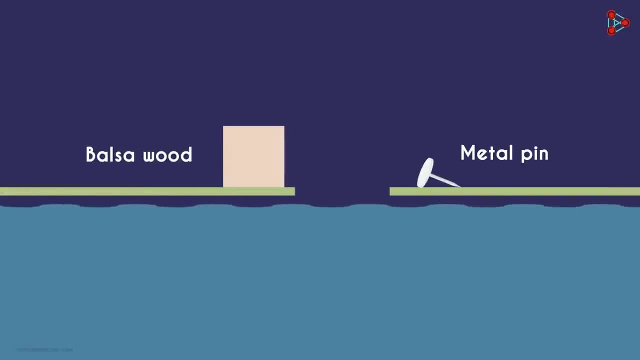 Now, let's say you simultaneously drop a piece of balsa wood and a metal drawing pin of the same mass into a container filled with water. What do you think will happen? Will both of them float, Or will they both sink, Or one stays afloat and one sinks? We will understand this example in the next video. 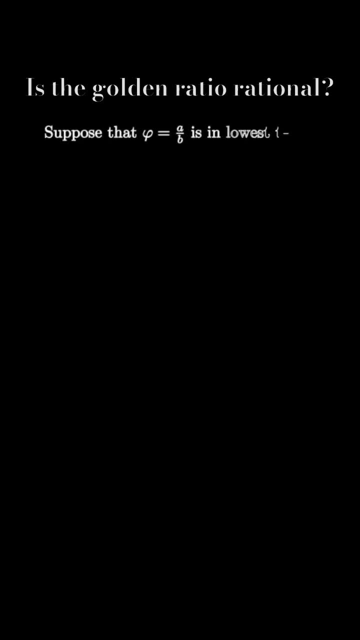 Suppose the golden ratio were a rational number, That means we could write it as a over b, where a and b are positive integers, and this is in lowest terms. The existence of two such integers means that we can draw this regular pentagon with a diagonal of length a and a side. 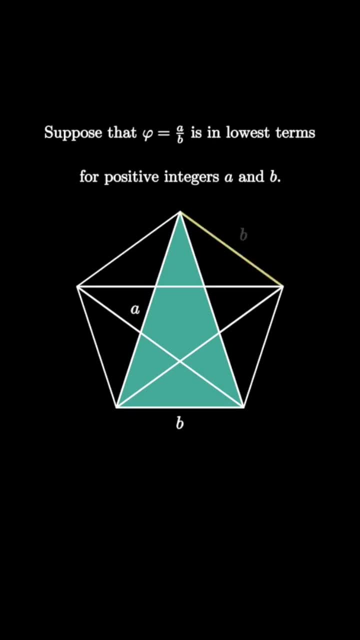 length of b, The pictured green triangle is known as a golden triangle. When we swing this side length down into the golden triangle, we create a second triangle, pictured in red. that's also a golden triangle, with corresponding side lengths b and a minus b. But because these two triangles 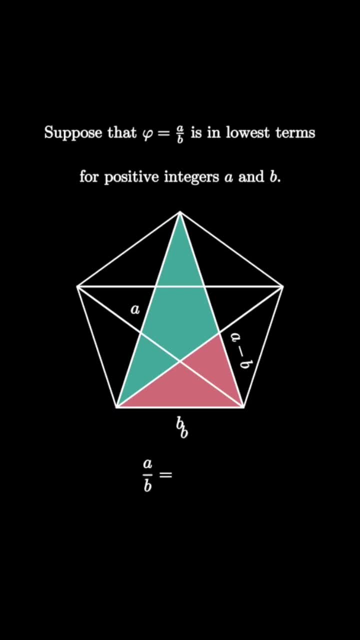 are similar, that means that a over b is equal to b. divided by a minus b, This means that the golden ratio, phi, is equal to b over a minus b. but that's a contradiction, since b is less than a and a minus b is less than b. so phi equals a over b. couldn't have been in lowest terms.